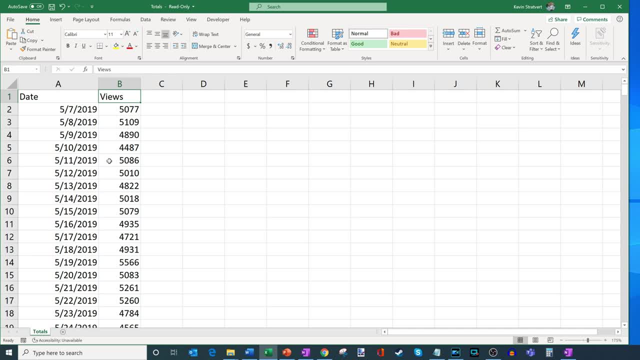 on this growth. can Excel help me forecast what the future looks like? And the answer is yes, Excel can do that. So what I'm going to do is: I'm going to go ahead, and I'm going to go ahead and do that. So how do we do this? Well, I'm going to show two different methods, or two different 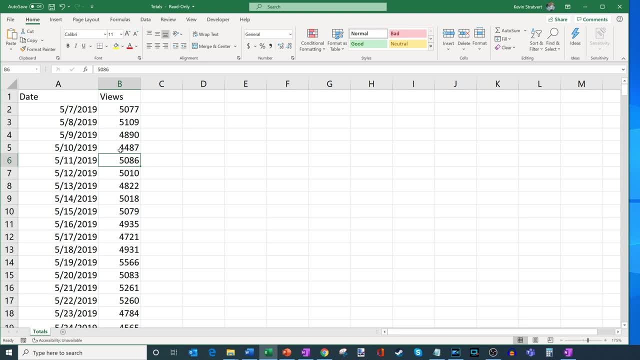 techniques that we could use to forecast. The first one is pretty simple, and this is one that I've used for a long time. What we're going to do is we're going to go up onto the pivots up here and we're going to click on insert And on insert. what we want to do is we want to insert a line. 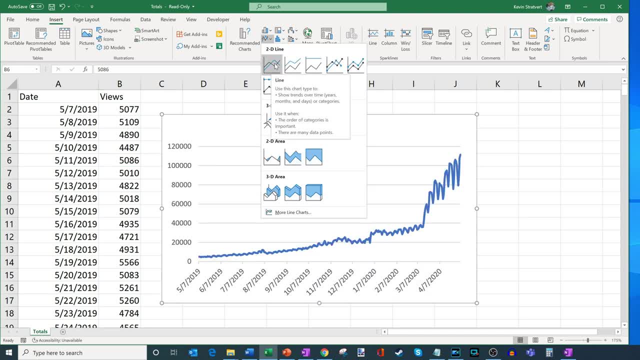 chart, And so I'm just going to insert a very simple 2D line chart, and let's go ahead and throw this in. So now this gives me a nice visualization of what the future looks like. So let's go ahead and throw this in. So now this gives me a nice visualization of what the future. 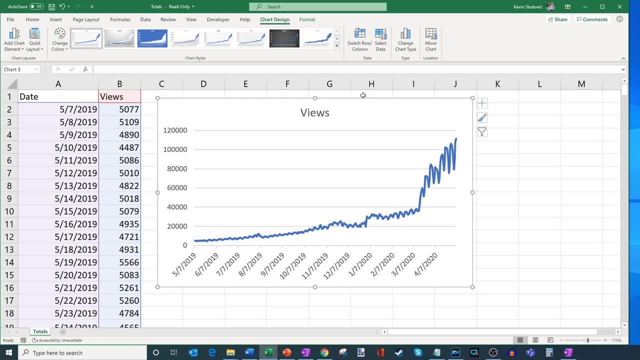 looks like, So let's go ahead and throw this in. So now this gives me a nice visualization of what my views have looked like over time. So it started out there was some growth, a little bit of growth, and then, especially recently, it's grown quite a bit more, And so this is what the past 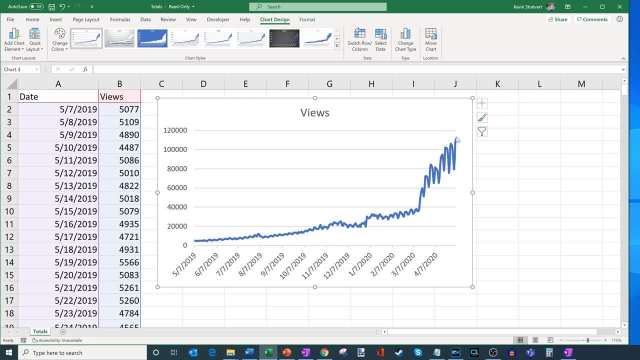 year looks like for me. And now to be able to forecast into the future, what does the future hold? What I can do is I'm going to just click on this line with my left mouse button, and now I'm going to right click on it, And what I can do here is I can add something called a trend line. So 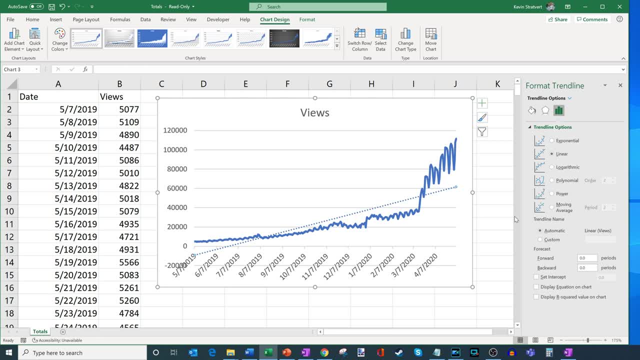 let's go ahead and throw that in, And within trend line I have a whole bunch of different options. We're going to walk through what all these different options mean and which ones you should use. So one of the things is: you'll see this trend line here and the trend line tries to match my data as closely as possible. 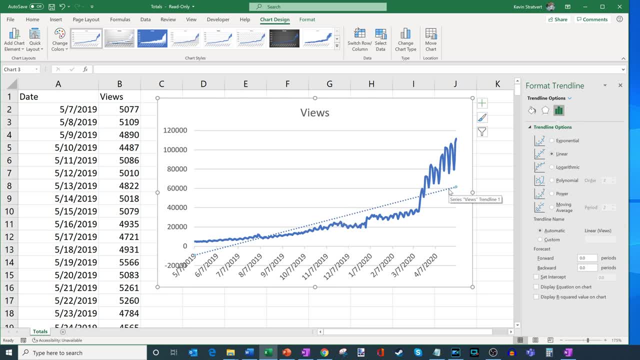 So, right now, the default is just a linear line or trend line, And so linear line is just a straight line, And this is the best attempt at matching the data. One of the things that you'll see, though, is it doesn't perfectly match the data. 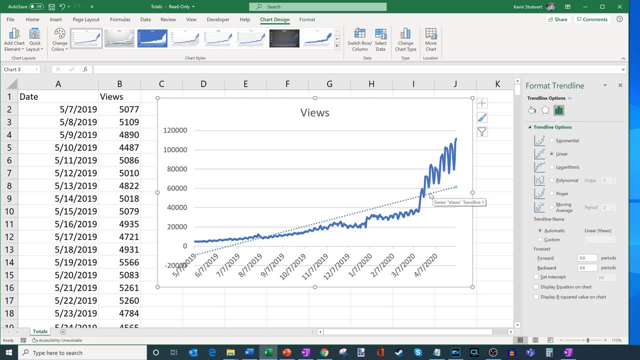 Here it's a little above, and then more recently it's below, So this probably doesn't reflect the growth accurately, And so I might want to try some of these other trend lines. So here I can look at an exponential growth line, And this one matches the data much more closely. Here it's pretty much. 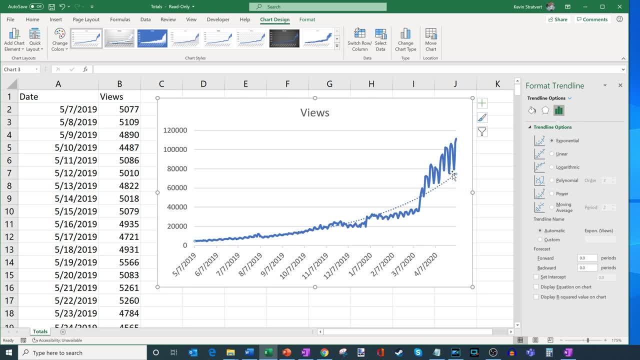 identical Up until recently. now it's a little below, But this one matches the data a lot better, And so perhaps on YouTube, growth is more exponential. as you grow, as you get more videos, The growth tends to be more exponential in nature. 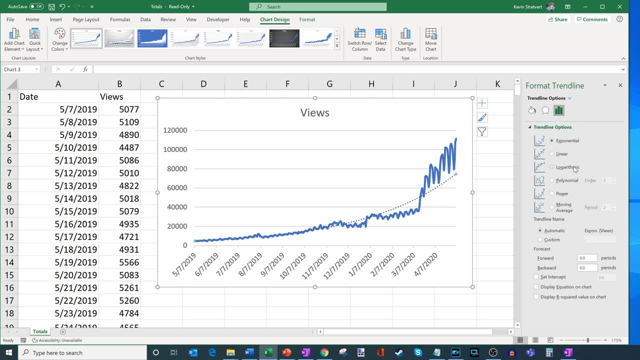 But what I can also do is I could click into different trend line options and see which ones match my data. So here's a logarithmic. I could also look at polynomial And then you could adjust the numbers here. So this one here. this is close to the data performance. So I could go through. 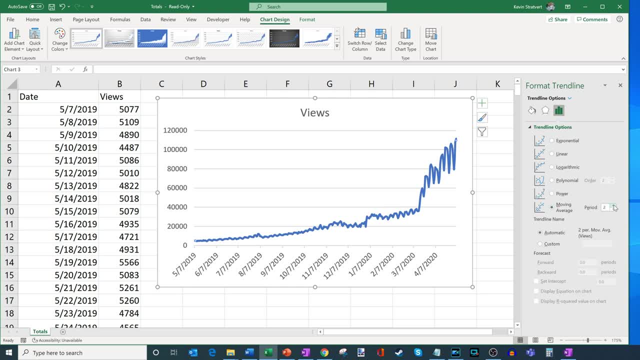 it. here I could also look at power, And then you could also do a moving average. So here I could say, hey, give me a moving average, say over a 20-day period. So this is different ways I could look at my data. 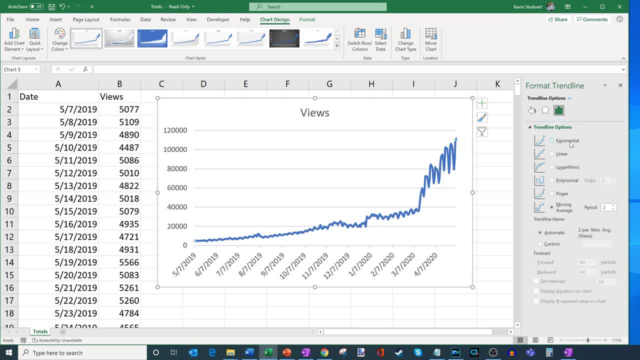 What I think. probably, at least going through these different ones, the one that appeared to match my data the best was this exponential line, So I'll go ahead and choose this. Now, some of the things that I can also look at is there's something called an R-squared value. I'm going to go ahead and click on this, And what? 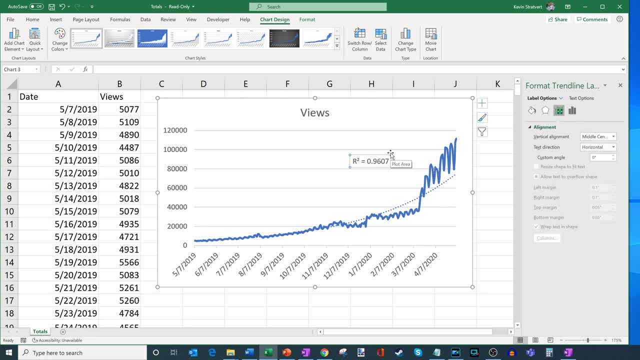 that stands for. this is the coefficient of determination, And it's a value between 0 and 1.. In essence, if it's closer to 0, that means the line doesn't match your data that well. The closer to 1 you are, the more closely that the line matches your data. So I'm going to go ahead and 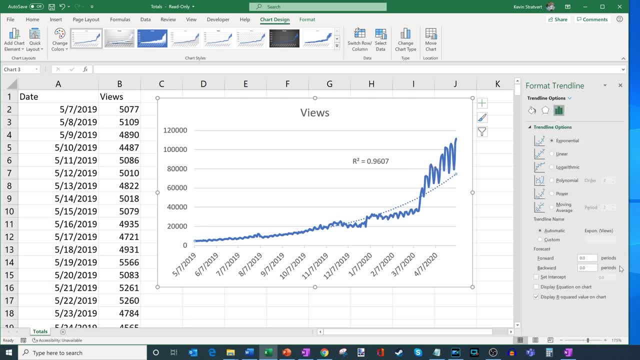 choose that, And so here I could go back to the trend line And I can click through these different options. So here with a linear line, it's a 0.7.. So really it doesn't match the data as well, And I. 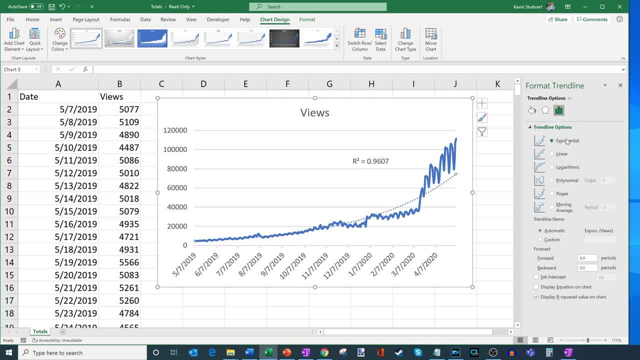 could go through and I could see how it matches the data, But here exponential seems like the best match, So I'm going to go ahead and choose that one. So now I mentioned that we want to do forecasting And so to forecast. what I want to do is I'm going to scroll down here And here you. 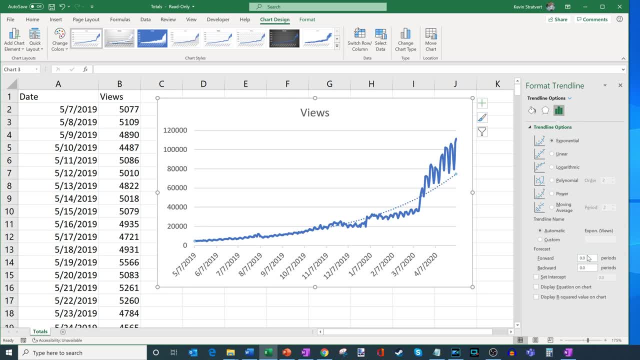 see a section called forecast, And so you could forecast both forward and backward, And so I'm going to go backward And what I want to do is I want to forecast into the future to see what things might look like, And now it says zero periods. What is a period? Well, my data in the spreadsheet. I go. 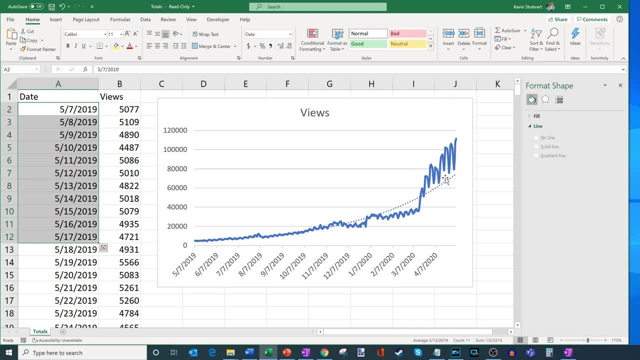 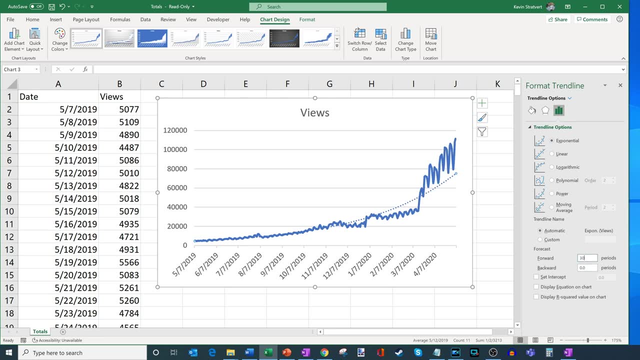 day by day by day, And so a period. then, if I click back in one period would be one day. So here I'm forecasting one day into the future. Here I could forecast 30 days into the future. So let's say a. 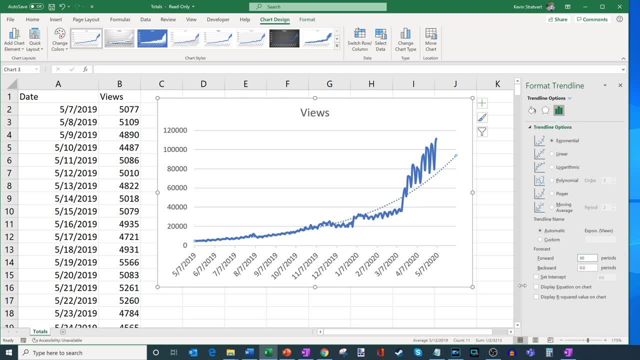 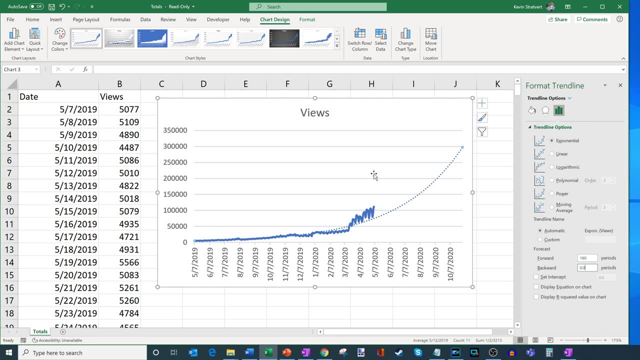 month into the future, And then maybe I want to even say, let's say 90 days into the future, So about three months. And then maybe let's say a month into the future, And then maybe I want to say half a year from now, So about 180 days from now. What this will do is it shows me approximately. 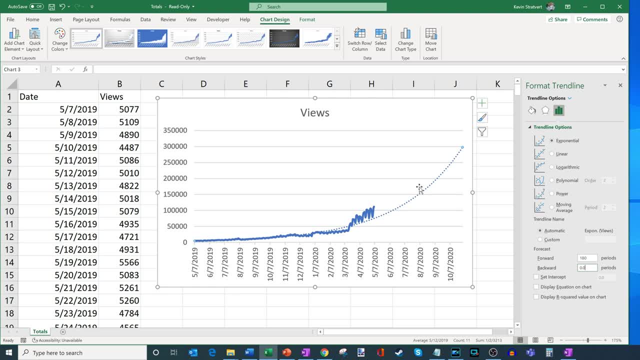 assuming that I do have exponential growth on the channel, This will show approximately where I would be in about a half a year. So here it's predicting about 300,000 views. if I look at it here Now, one of the big questions is: is it exponential growth or does it actually tend to be more linear? 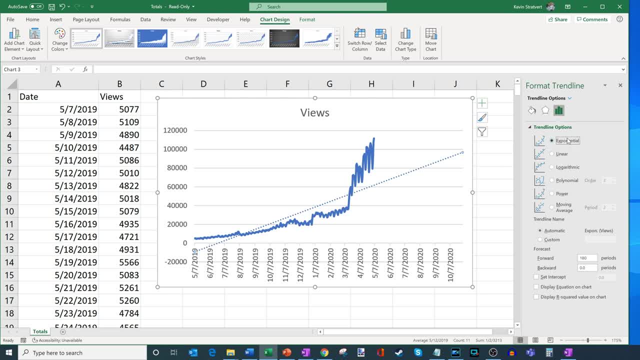 If it's more linear, I'll be at about 100,000 or so. So it really depends on what type of trend you're in. I'll be at about 100,000, you know what's the value of your day, what's the value of? 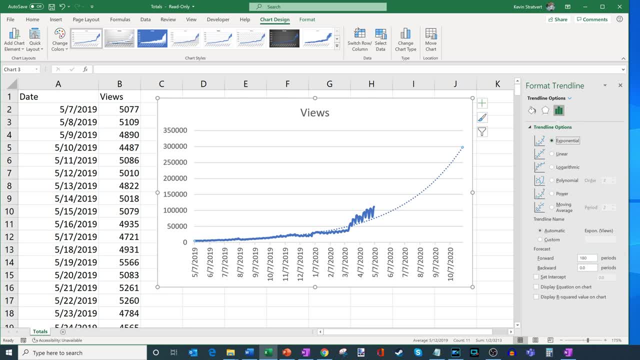 your week. what's the value of your month? what's the value of your month? And it's really going to depend on what you're doing in that day. So I'll be at about 100,000 in a month, 100,000 a year if 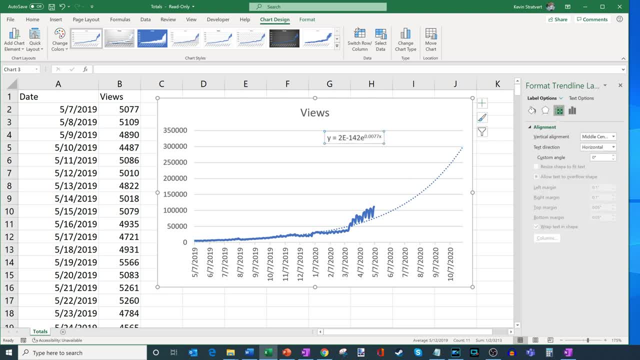 it's more linear, and then I'll be at about 100,000.. So this is where my forecast is going to be. So I'm going to be at about 100,000. so that matches your data And one of the things that's. 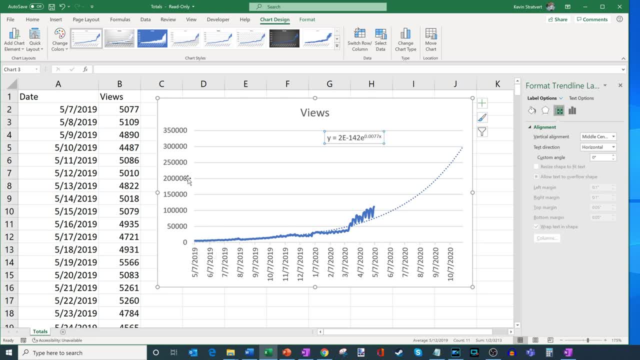 also interesting. so here I'm forecasting forward. what I can also do is I can display an equation on the chart, And so here's my equation and the X value. So once again a little refresher course back from math class, and that'll tell me the why, how many views I will have. 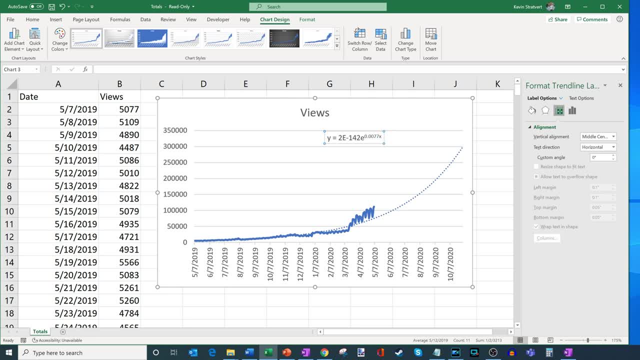 So that's another way where you can get the equation, and then you could simply type in your value and it'll tell you where you'll be at that point in time. Or, just as a simpler approach, you could simply type your number in here. 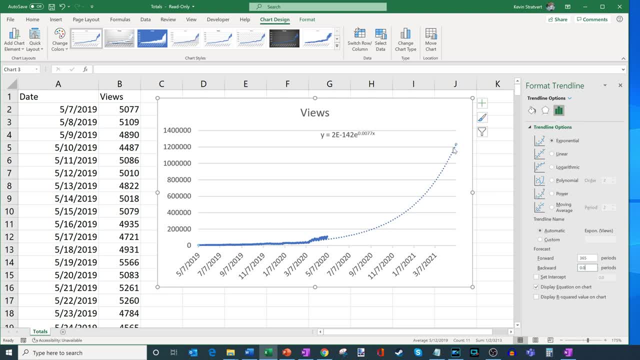 So let's say, a year from now, where am I gonna be? And here it's saying at about 1.2 million, Although, given that I've only seen this level of growth going another year in the future probably has a lot of uncertainty. 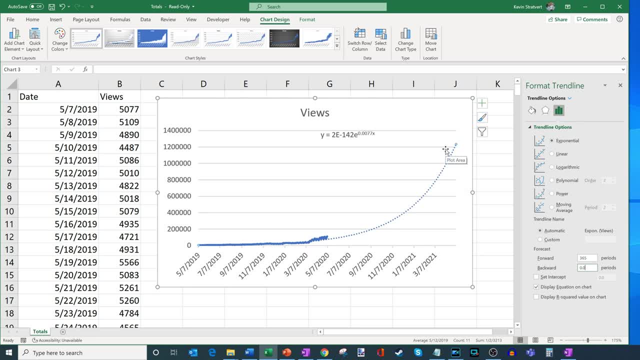 So that's one just quick way how you could add forecasting into charts in Microsoft Excel. And now I also wanna show you another way to do forecasting in Microsoft Excel. So I'm gonna go ahead. let's delete this for now. Here's my data. 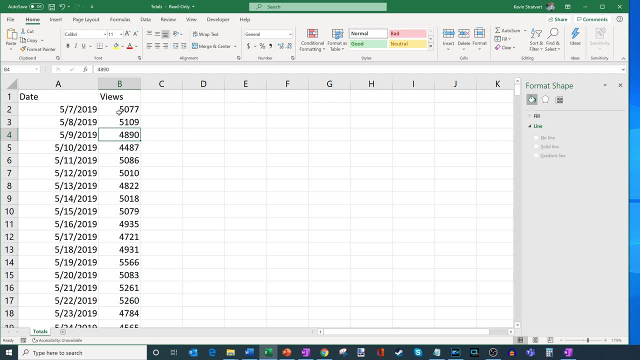 And what Excel has is they have a built-in dedicated formula or a forecasting view, And the way we're gonna get to that is we're gonna go up back up to these pivots across the top and we're gonna click into data. So let's click on data. 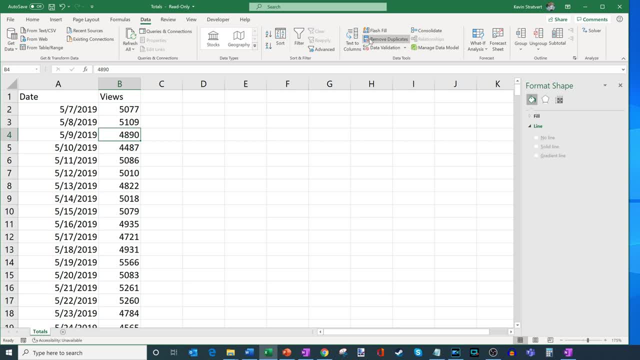 And then across the top here, one of the views here, one of the options on the ribbon, is called forecast sheet. So Excel has an entire sheet that'll help you forecast into the future. So let's go ahead and click on this, And this brings up a dialogue. now, 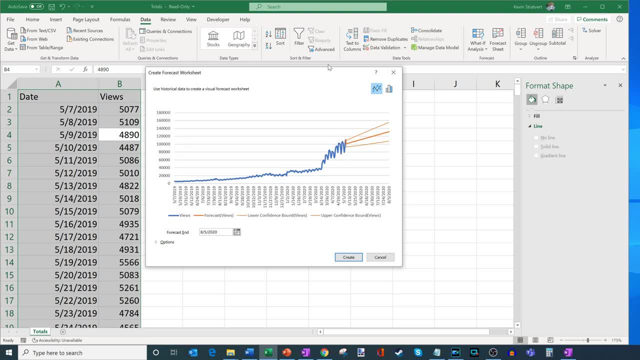 where it says create a forecast worksheet, And what it'll do is it'll use historical data to create a visual forecast worksheet. And so here's all my historical data of my views over time, And what it shows me then is it shows me the forecast. 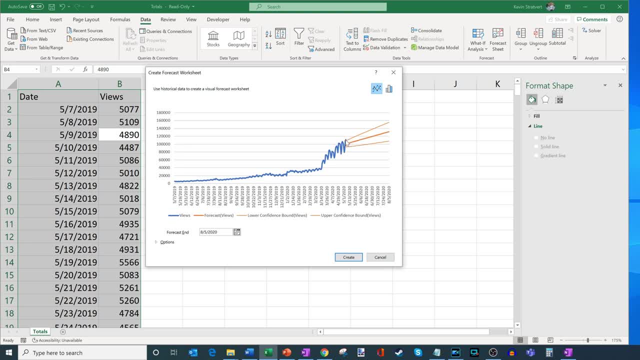 And value. here is this orange line, And then it also has an upper bound and a lower bound. So with 95% confidence, or 95% of the time, it's expected that the value would fall within this range. So something that I could see down here. 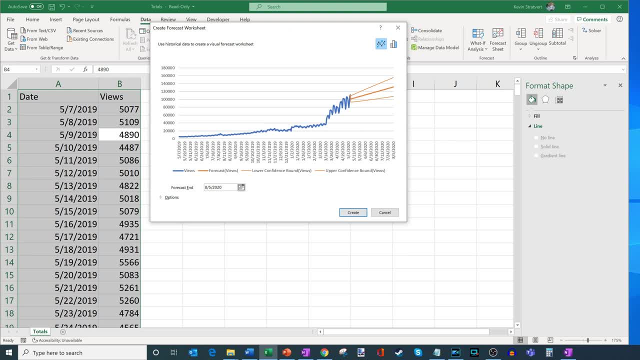 here I could see the forecast end. So here's forecasting through August 5th, So we're going about three months into the future. But I could also say hey, by the end of the year, where do I expect to be? 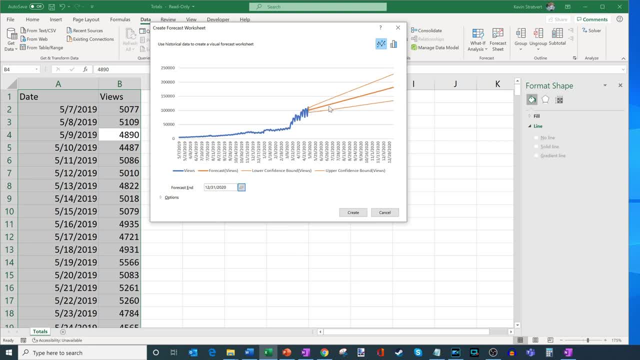 So I'm gonna go ahead and change the date, And so here's another view of of where it expects me to be by the end of the year. What I can also do is I'll click into options here, And here I could see when the forecast starts. 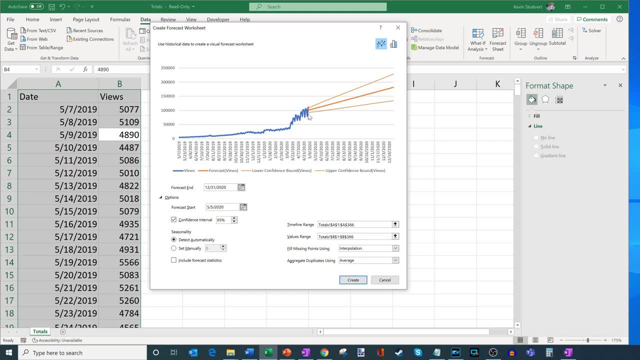 And so the forecast start date is basically the last date of data in my data here, And so it'll kick off there. I could also indicate the confidence interval. The more confident that you are, the wider the interval will get, as you see above. 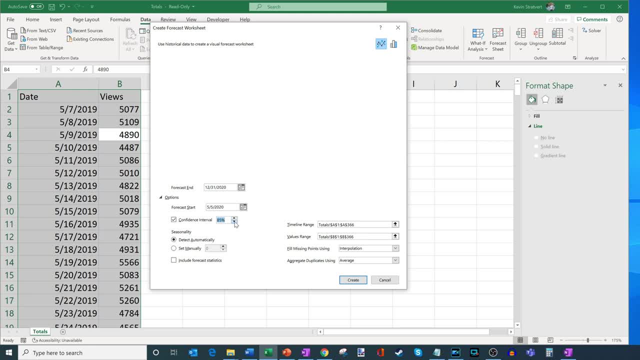 And the smaller it is. if I'm less confident, you'll see that the range narrows. So the more confidence the wider it is, the less confident the more narrow that it is. but I'll go at 95%. That's a pretty standard confidence interval percent to use. 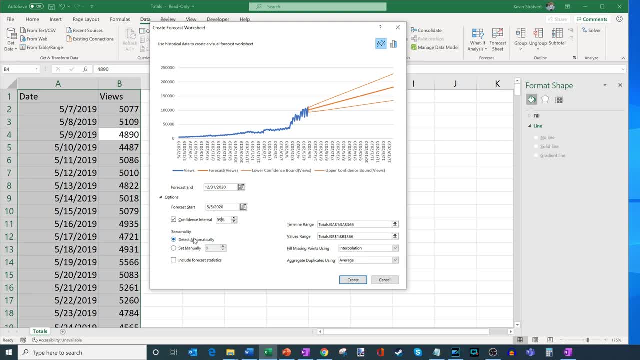 What's interesting too is if there's any seasonality in the data- So let's say on weekends it goes down or during the week it goes up- it'll detect that and it'll apply it to the forecast. I don't tend to have all that much seasonality. 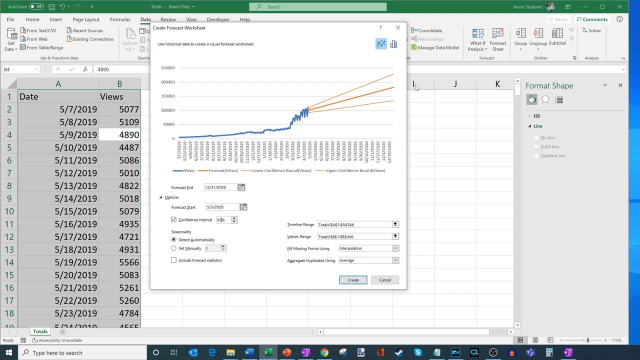 You have a little bit of seasonality on weekdays and weekends, but overall that doesn't affect this too much. You could also include forecast statistics And then also indicate: this is my timeline range, the values range, So it's just simply the data. 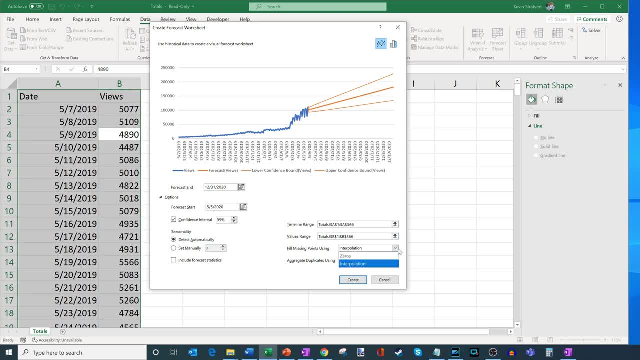 that I'm using from the spreadsheet, And then you could also fill missing points. So let's say I'm missing a few days here and there. You could either use zeros or interpolation, which will figure out approximately what the value would be And then also what you wanna do. 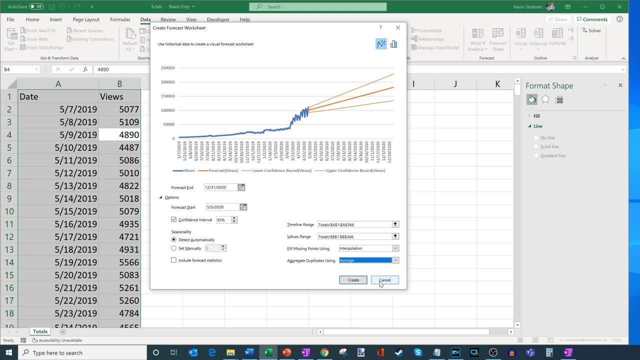 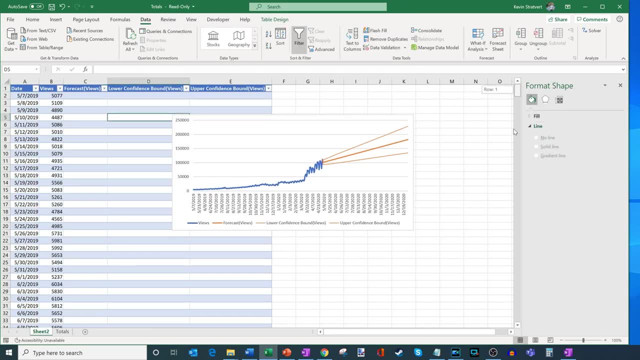 with any duplicate values in the data, And so what I'll do now, all of that looks good to me and I'm gonna go ahead and create the forecast sheet. So what it does is it creates a new table with all the. So what I'll do now, all of that looks good to me and I'm gonna go ahead and create the forecast sheet. So what it does is it creates a new table with all the. 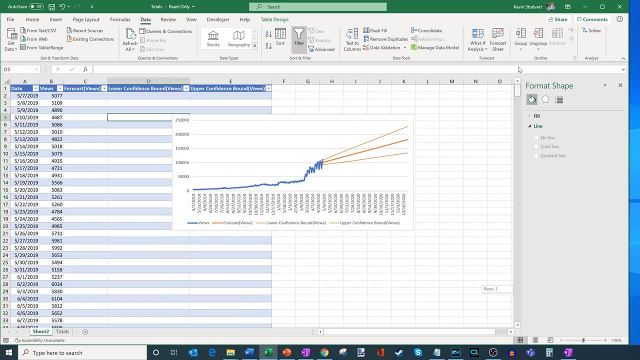 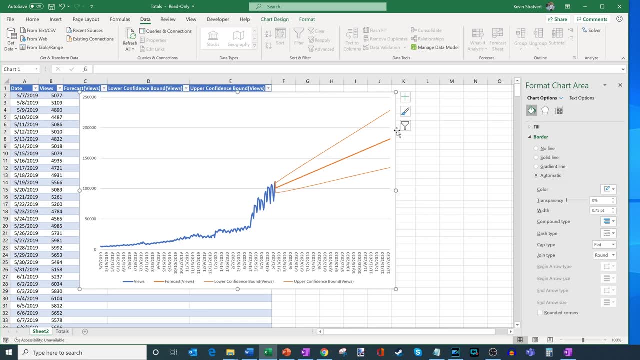 forecast data. So here, if I scroll down, I could see all the forecast data in table format. And here what it's done is it's created a nice chart for me that shows what the forecast looks like, And here this is through the end of the year. 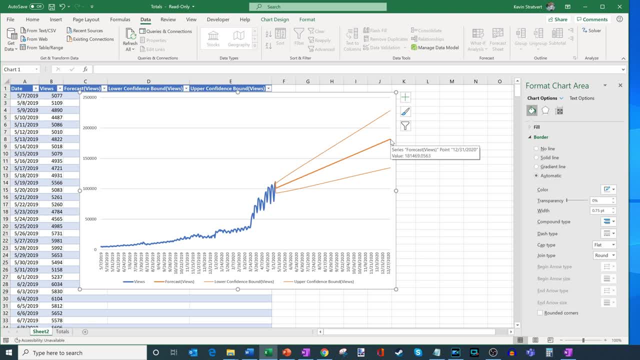 It's expecting that if I keep up the current growth rate, I'd be at about 181,000 views or anywhere between 230,000 approximately and 135,000.. So it expects or forecast the views to be within that range, to be within that range. 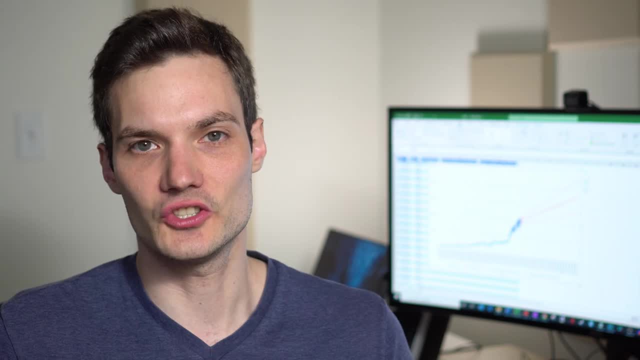 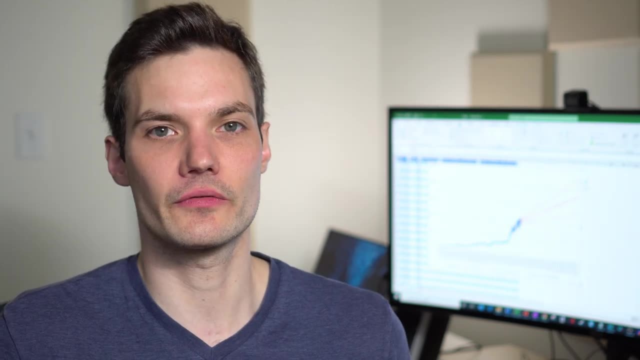 All right. well, that was just a really quick look at two different ways you can forecast in Microsoft Excel. You could either insert a chart and then you could forecast forward, or you could use forecast sheets and Excel will take care of most of the heavy lifting for you. 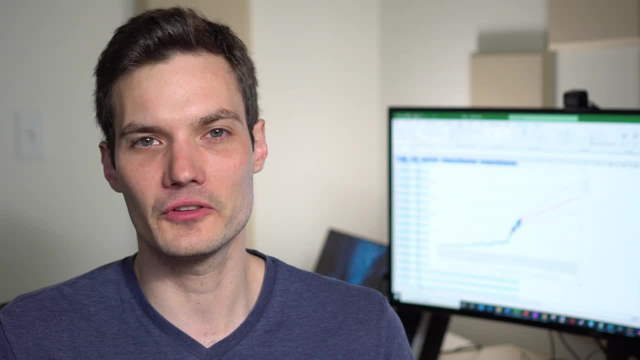 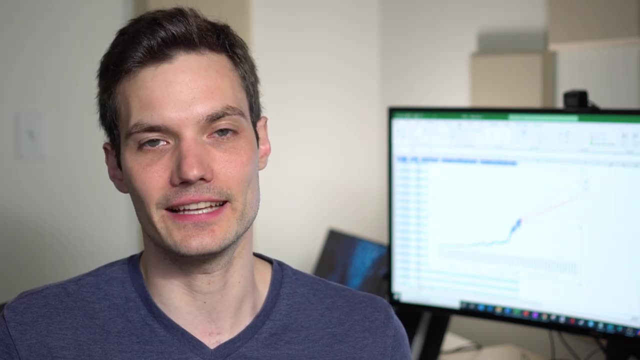 Either way, it's a kind of fun way you could predict what the future might look like with some amount of confidence. And of course it's always hard predicting the future. but if you use past data, that's your best indicator of what the future might hold. 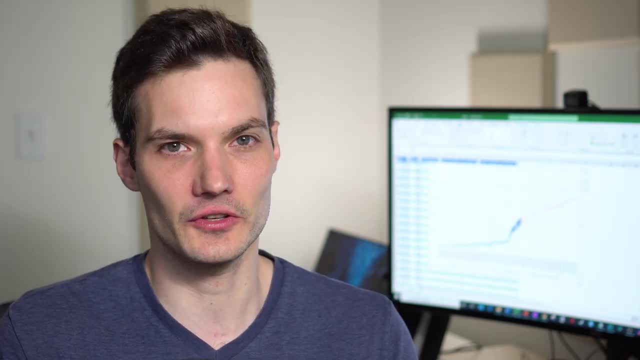 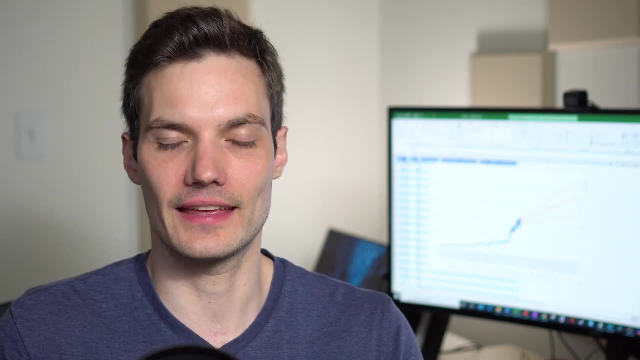 Anyway, if this video helped you learn how you could forecast into the future, please give this video a thumbs up. If you wanna see future videos like this, hit that subscribe button. That way you'll get a notification anytime new content like this comes out. 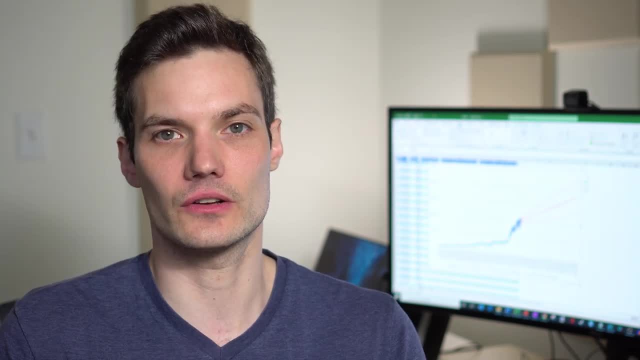 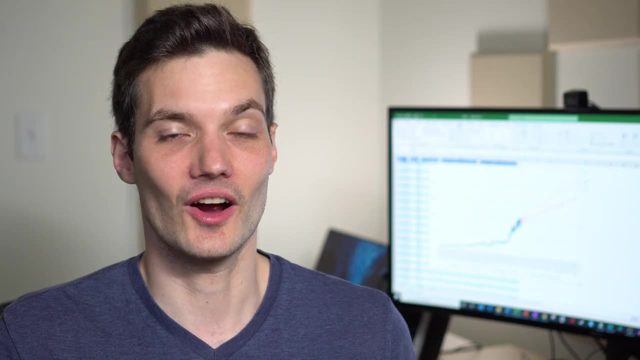 And, lastly, if there are any other topics or any other videos that you wanna see me cover in the future, simply leave a comment down below and I will add it to my list of videos to create. All right, well, that's all I had for you today.